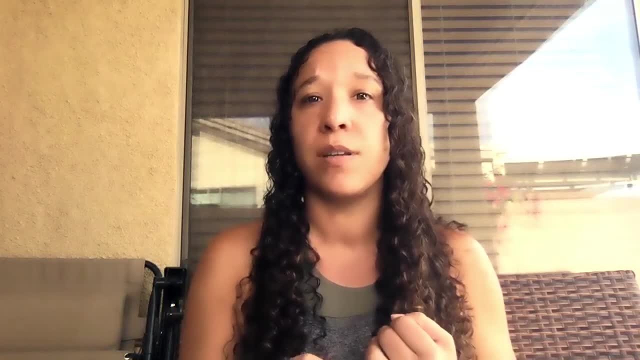 it can tell you why a child's engaging in a behavior because, in order to conduct baseline probes, you're going to be observing it And, as a trained behavior professional, you're going to be able to notice the antecedents and the consequences. 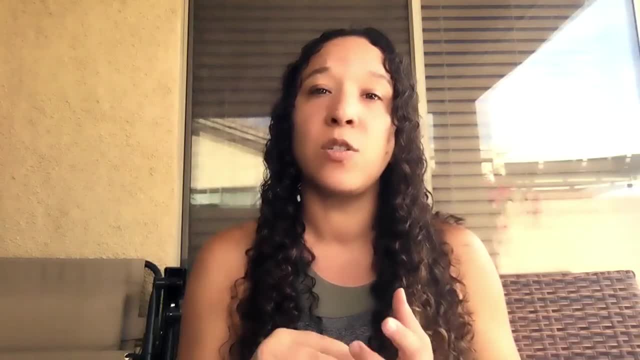 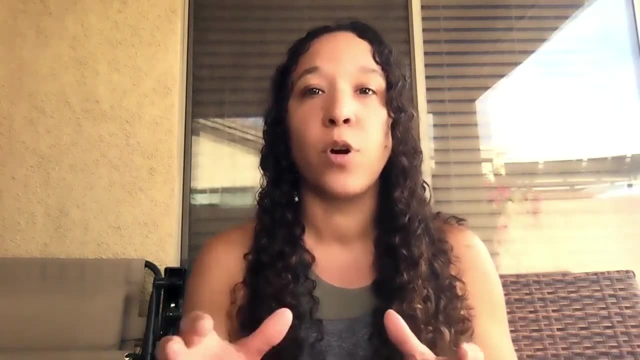 That are maintaining it. The other thing you're going to do is you're going to be able to use the information to determine the intervention. So, for example, you might be able to determine the levels of reinforcement required, because if you set the reinforcement bar too high, 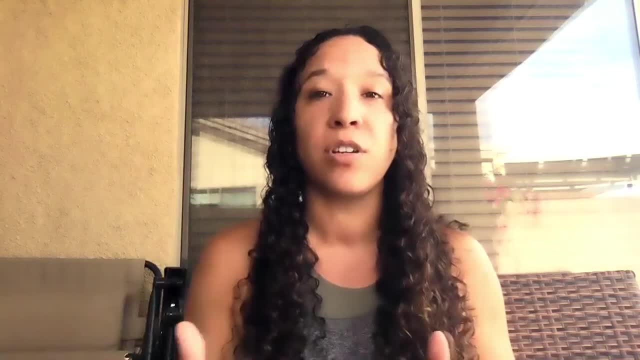 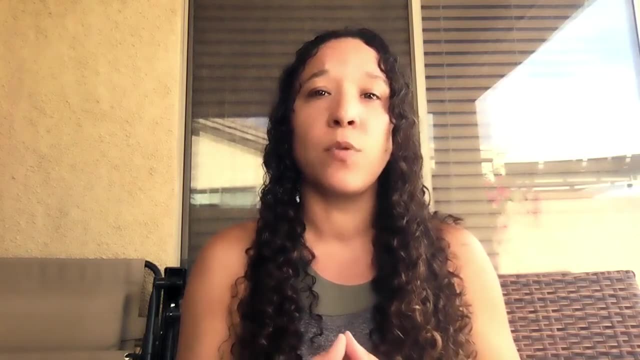 the child may not get access to reinforcement and intervention and the intervention may not work. The third thing is sometimes you find out when you're conducting baseline probes that a behavior really doesn't need to be intervened upon. So, for example, I was recently conducting a baseline probe for a child. 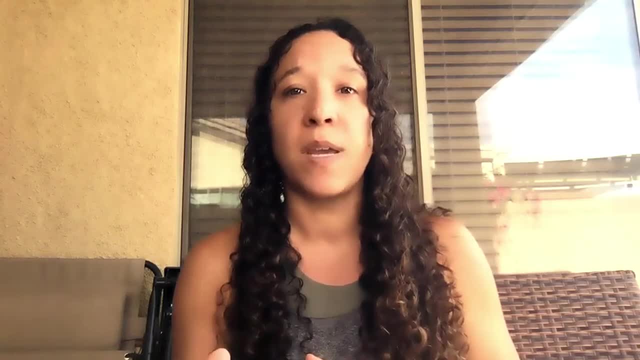 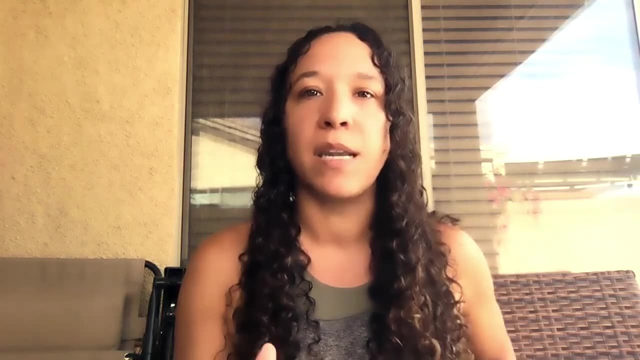 that would scream but it when I was conducting those baseline probes I actually found out it was caused by an extraneous variable in the environment and it was not occurring at a rate high enough that we needed to intervene with it. And once we're able to fix that extraneous variable, 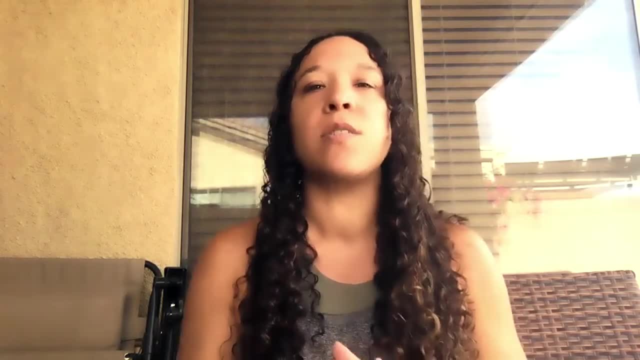 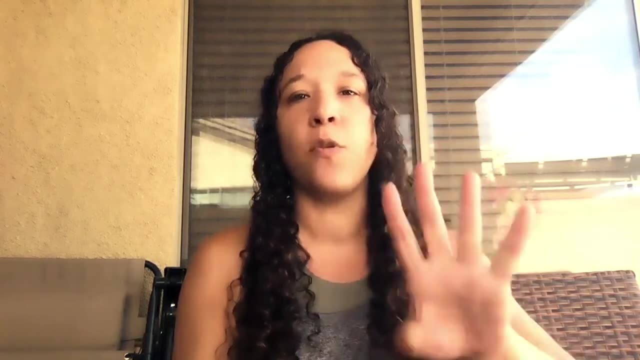 which was a really easy fix. we actually didn't need an intervention, So sometimes baseline can give you a lot more information than you would think. So once you're conducting a baseline, there's going to be four different ways the graph can look. 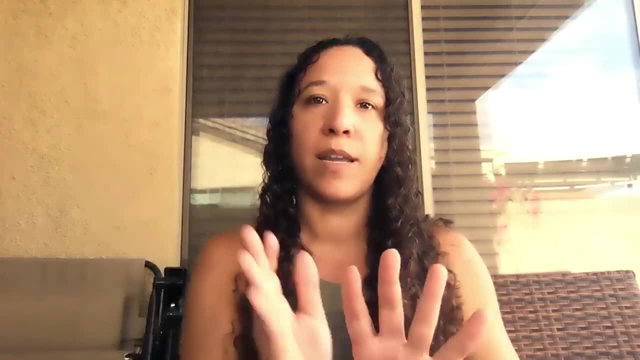 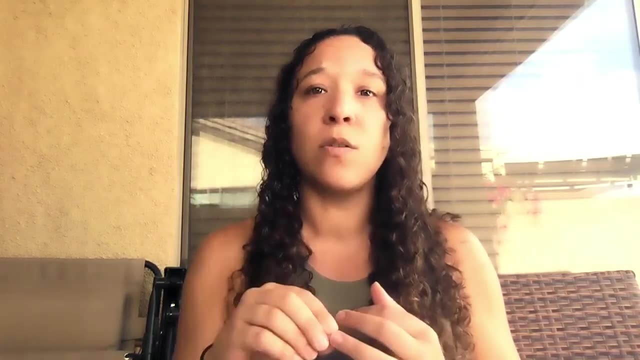 And obviously we're going to be visually graphing the baseline data, right? So sometimes the data looks like it's ascending. If that's the case, it means that the behavior is increasing. So if it is a behavior you don't want to see, 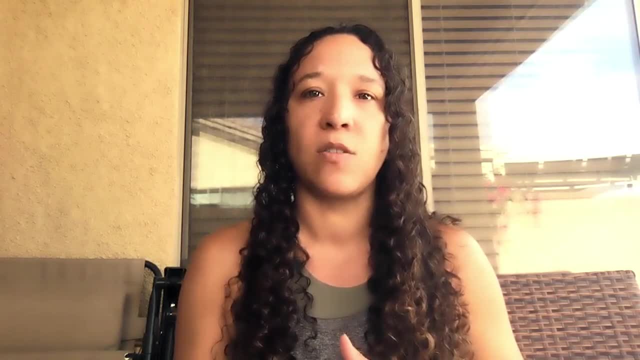 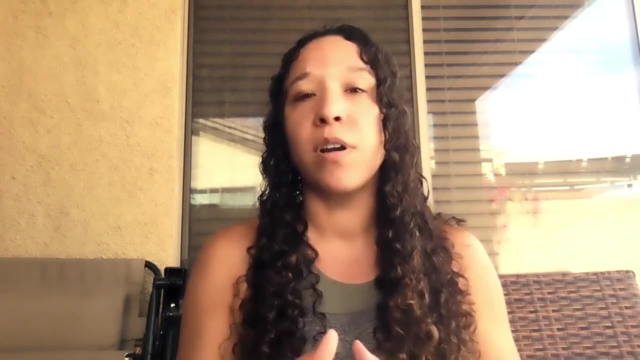 it may be an indication that you don't want to wait for a stable baseline to intervene. You want to intervene right away, especially if the behavior is dangerous or self injurious or really causing harm to the child, Or if it's a behavior you do want to see and it's increasing. 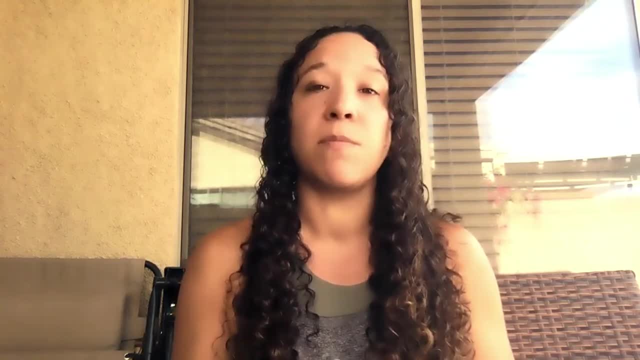 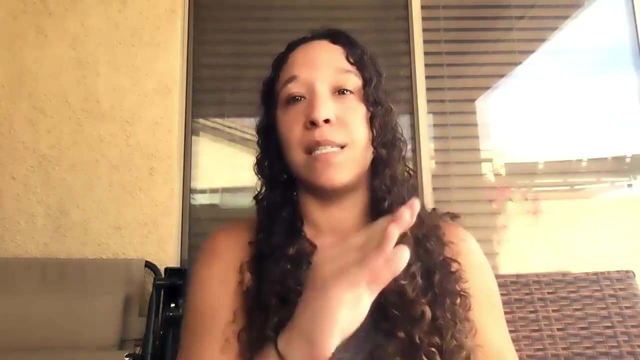 that means you might not need to respond and you might not need an intervention, because it means the child is already acquiring the skill. So the same thing holds true for the second condition, which is decreasing. If the behavior is decreasing, if it's an important skill for that child, 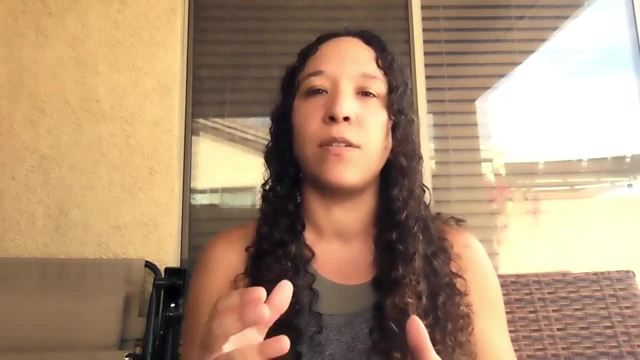 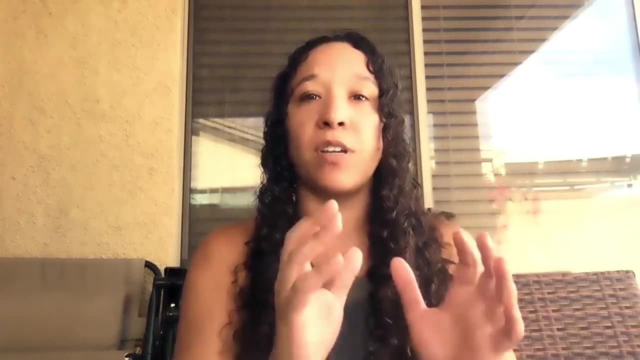 you may want to intervene right away. I tend to lean on the side of ethical, ethical considerations of what's best for the child, not what's best for research. So for me I would intervene right away. But if again the behavior is a behavior you don't want to see and it's decreasing on its own, 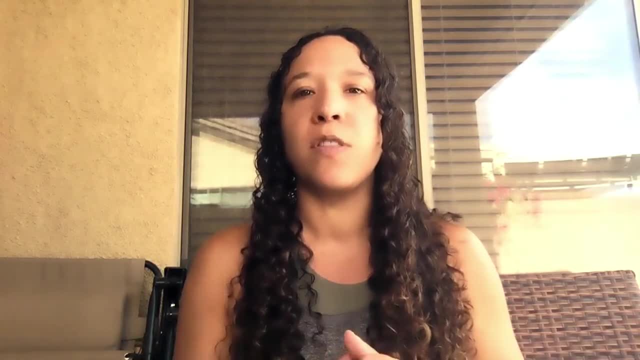 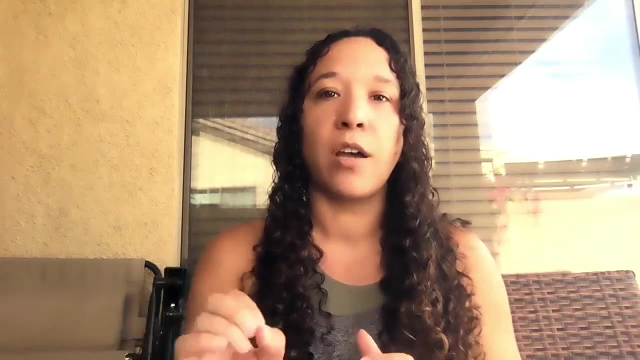 you again may not need an intervention. The third thing would be if the behavior occurs at a very variable rate. So that would be the behavior that I saw when I was collecting baseline data on this child who was screaming. it either happened a hundred times per hour and 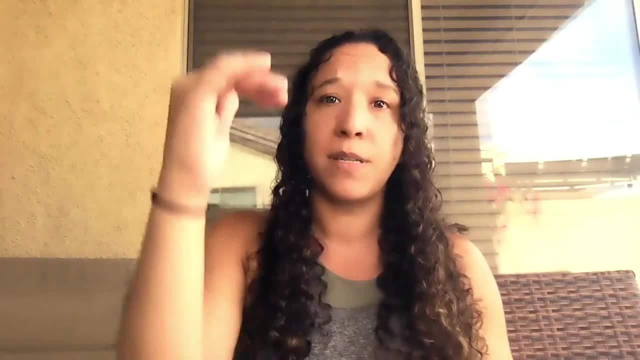 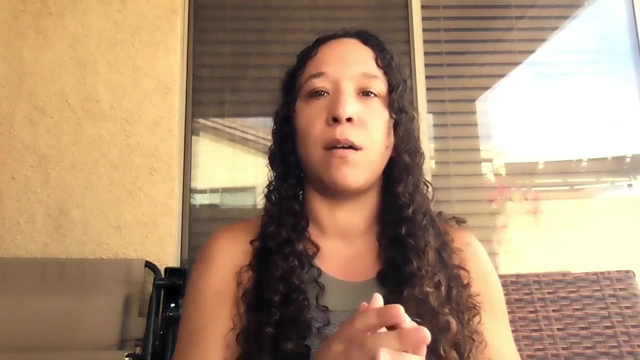 or it happened no times per hour, right, And it was up and down, and up and down, and up and down, And that made me realize, okay, wait a second, here's something in the environment that's triggering this behavior. This is not necessarily something we need to create intervention for. 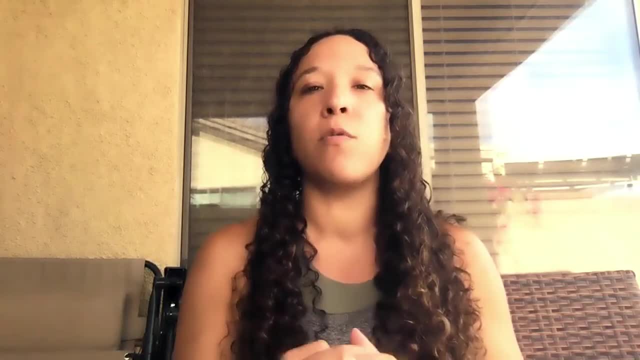 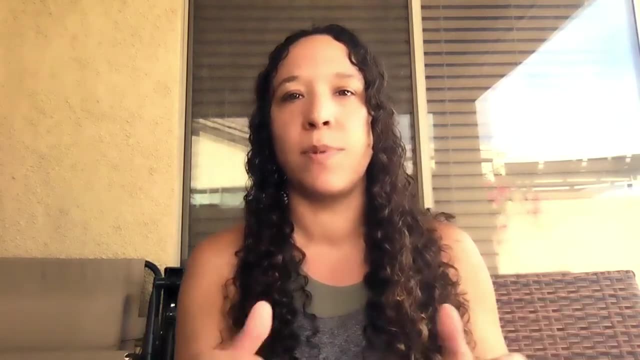 We need to figure out: why is the child doing this? The fourth thing would be: the baseline is stable. Now this is when, typically, you should always intervene. You always want to intervene when a baseline is stable, because once you have a stable rate of responding, then you have a control. Okay, 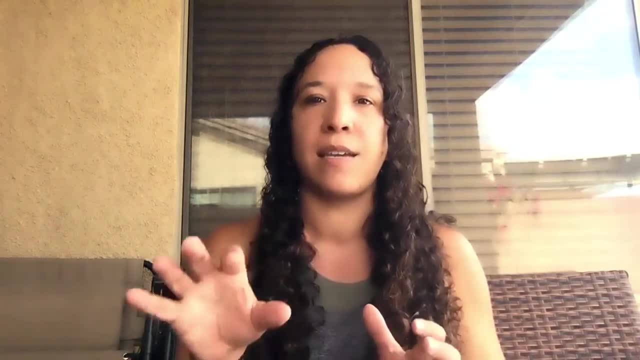 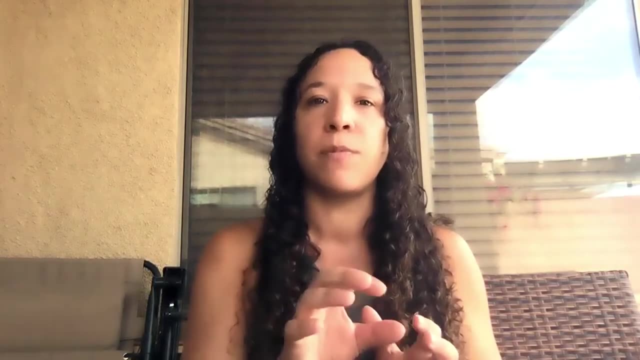 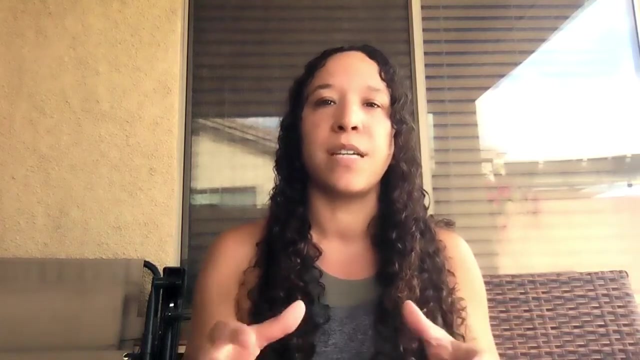 So now, what would you do once you established a stable baseline? What do you use that baseline for? Well, you're going to use that baseline to create a functional relationship or demonstrate experimental control when implementing an intervention. So there's going to be four parts to that. The first part is prediction. 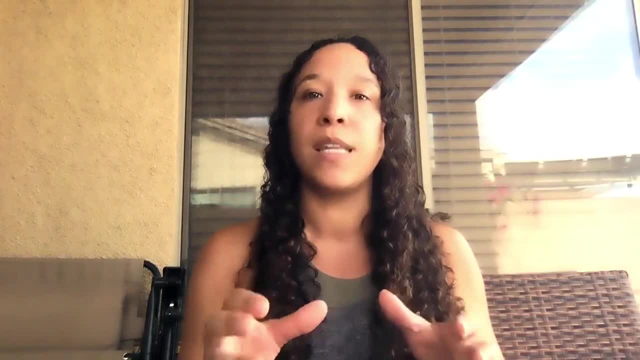 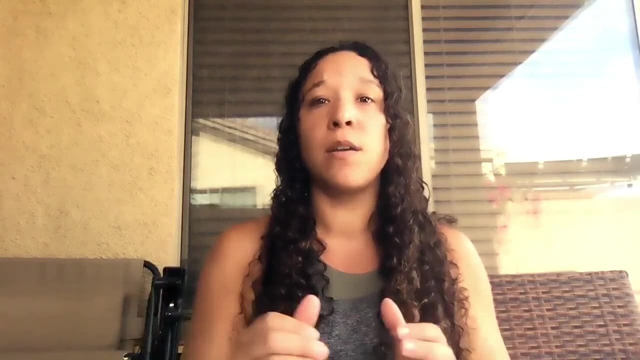 Prediction simply says that you predict or you believe that future behavior would occur at the same rate if you did not intervene, which makes sense, right? So you make that prediction. Well, how do you prove that prediction? Well, it's called the next part. 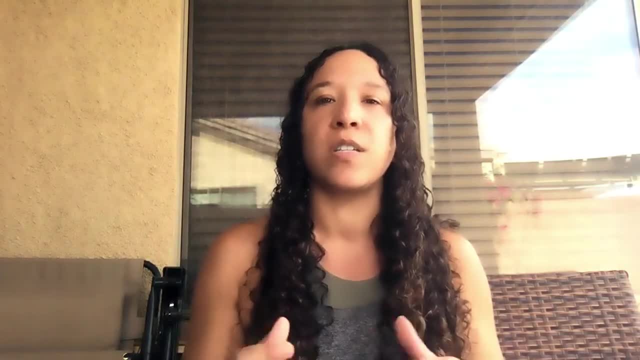 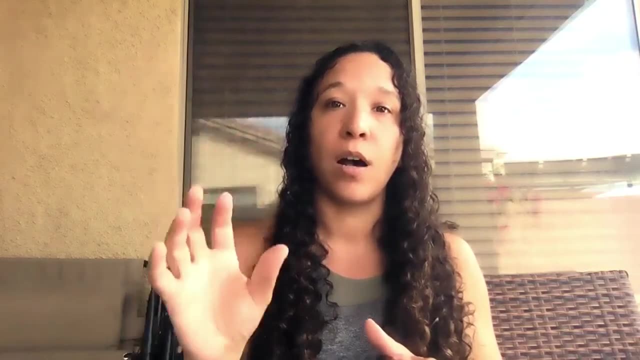 You would put the intervention in place and it's called affirmation of consequent And essentially what you're doing in that phase is that you're demonstrating that the intervention- again the independent variable- caused the behavior change- a dependent variable. So if you see that the behavior continues to stay the same, well, 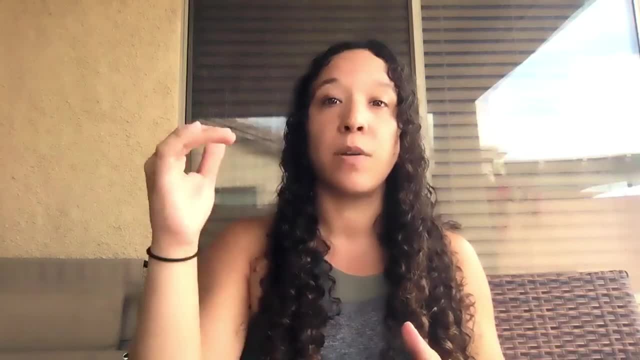 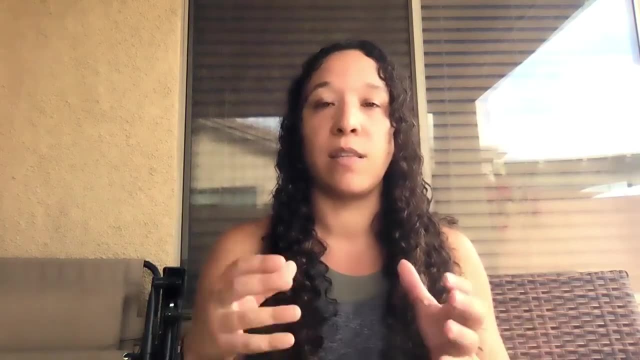 then the intervention didn't work. but let's say, the behavior increases, if you want it to increase, or decreases, if you want it to decrease. then you can demonstrate that the prediction was accurate and that the intervention worked right. So what do you do now? Okay, You prove this. 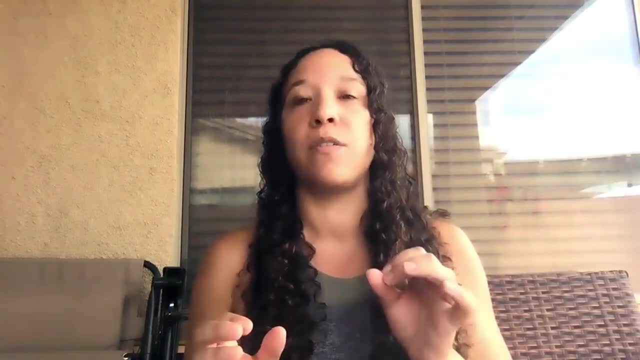 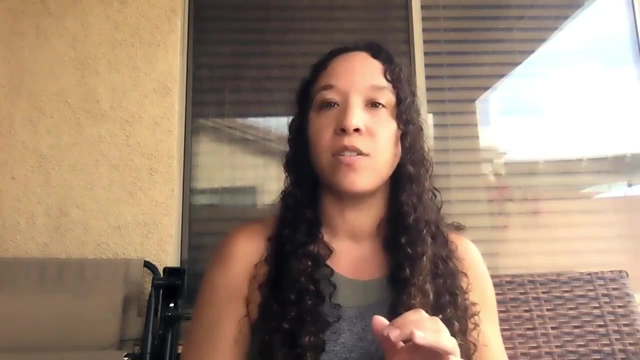 The next step you want to use is: you want to verify- it's called verification- that you're correct, And the way you would do that is returning to the baseline. You would withdraw the intervention and return to the baseline. Now, this only works with a behavior that is not learned. So, for example, 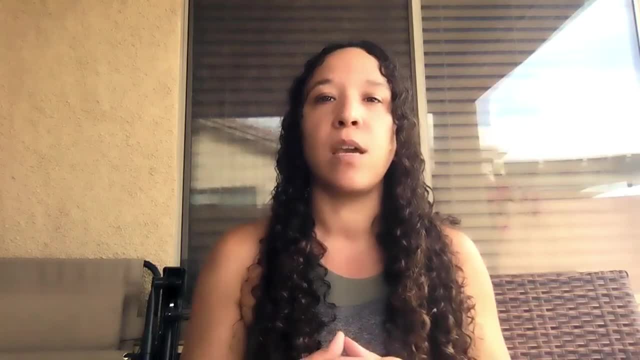 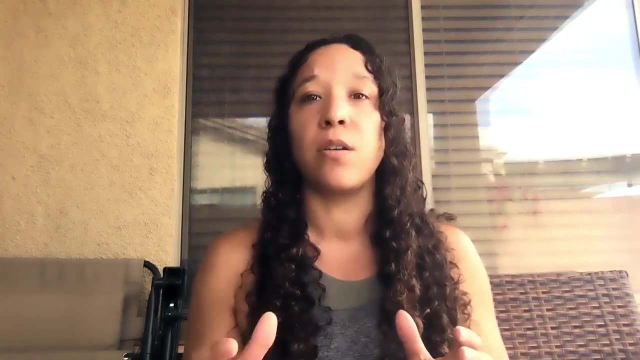 if you're using an intervention to teach a child to tie his shoes, then you can't withdraw it. expect they're going to stop tying their shoes once they learned to tie their shoes, But in the in the case that a behavior is unlearned, the 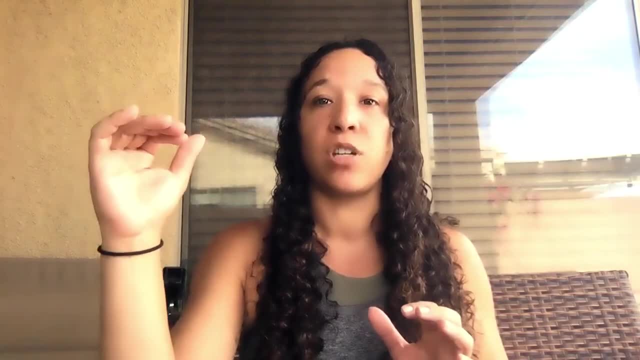 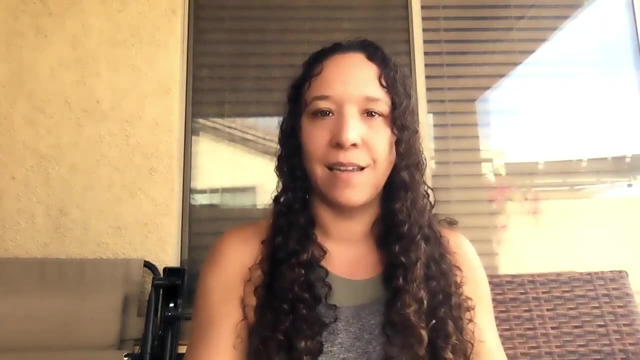 if the intervention truly was what was creating a functional relationship to the dependent variable, the behavior, the rate of responding should go back to baseline. And then what are you going to do? You're going to replicate it. That's the third, fourth base replication. 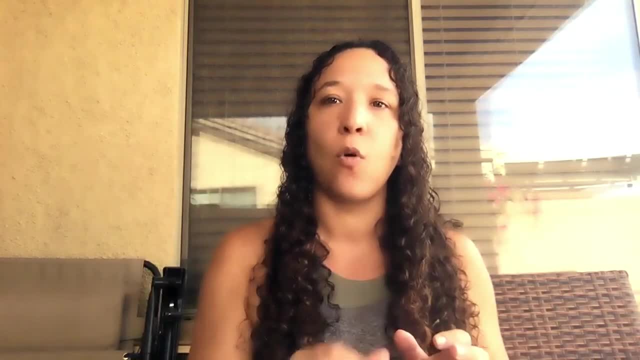 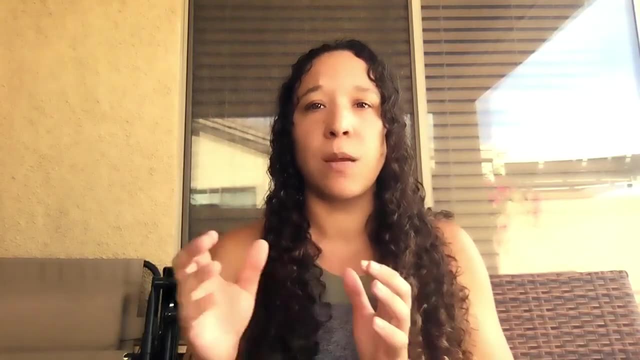 essentially putting the intervention back in place, And does the rate go back up or go back down, depending upon what you're looking for it to do? Now you can do this multiple times. The more times that you do this, withdraw the intervention and put it back. 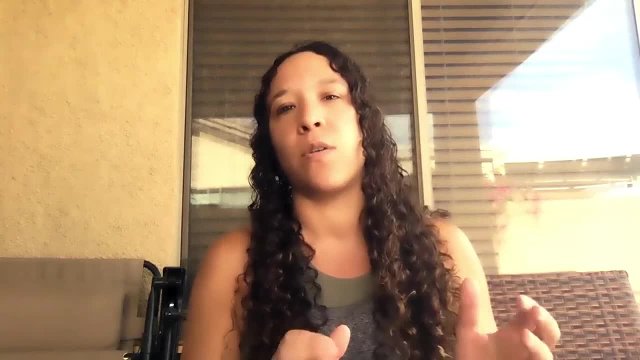 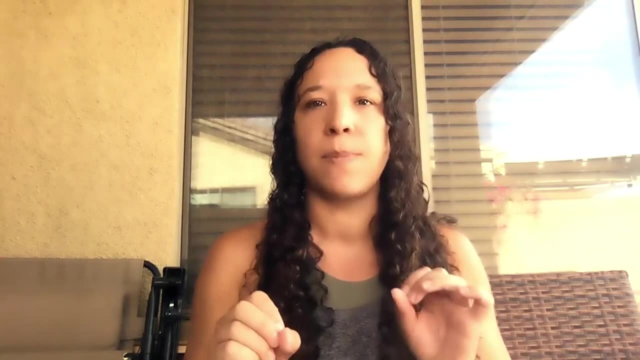 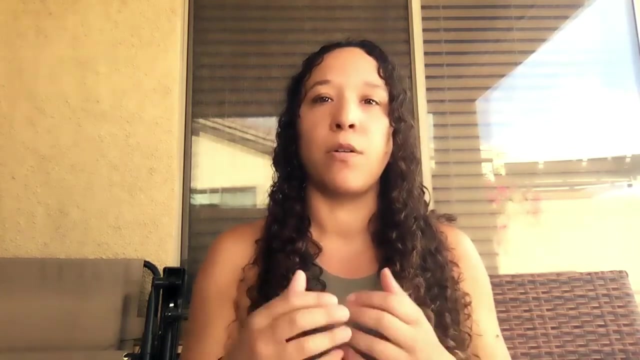 the better the functional relationship is. Now, I alluded to ethics earlier. There are some people who think that this is the most ethical thing to do, because it really demonstrates functional relationships that were science-based and that experimental control is important to prove. I tend to believe it's unethical and a lot of people are believe this. 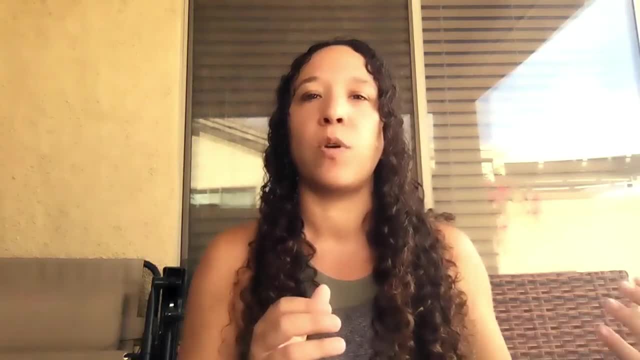 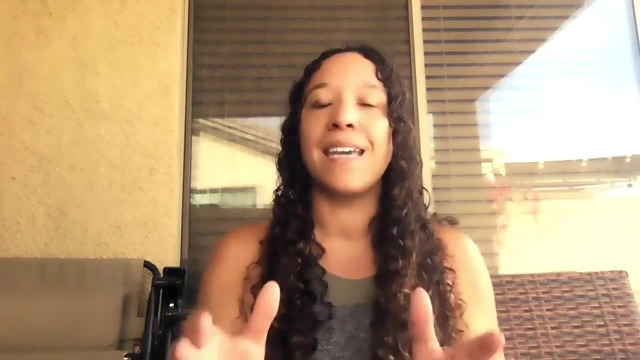 especially people in ABA today, as opposed to ABA 15,, 20 years ago, that it's not ethical to withdraw an intervention that's working for a child, just to prove functional relationship. I tend to be of that camp. I believe that, rather than you know, you withdraw an intervention. 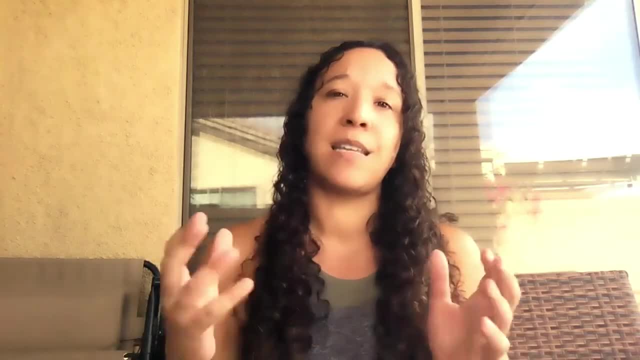 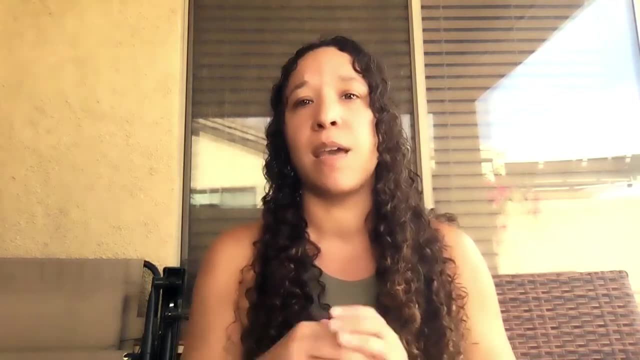 you should show it across. multiple people, multiple settings. I tend to like a multiple baseline design as opposed to withdrawal design, but that is something you need to decide for yourself. as a BCBA, It is considered ethical to withdraw an intervention, In fact, 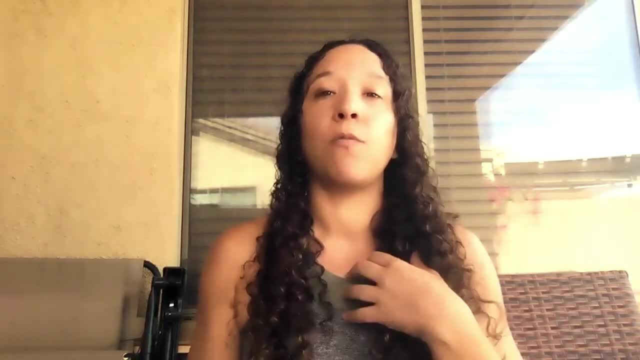 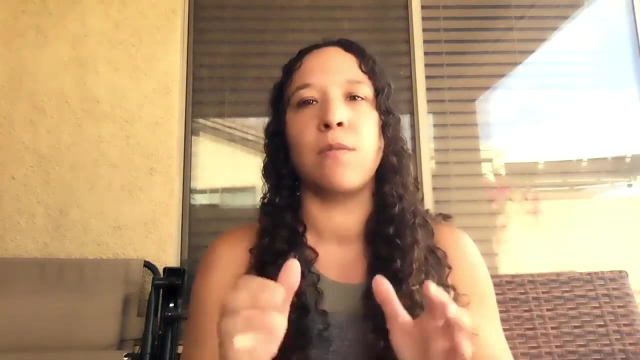 it's considered recommended. It is not something I personally, ethically, would do, Um, and that's just my personal choice. So this is, though, of everything you need to know about, a baseline we did cover in this video, So I really do hope you found it helpful. Again, I'm traveling. 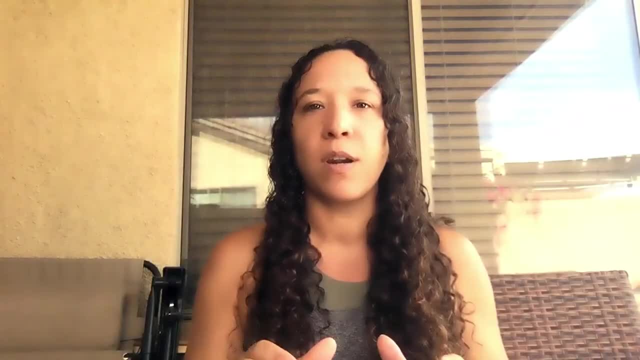 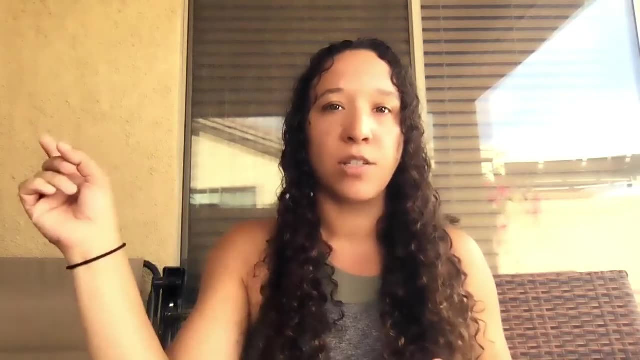 so I'm about to go hiking. pardon the casual appearance, but I really wanted to get this video out for you this morning. If you found it helpful, if you appreciate me getting up early to put this video out for you, subscribe to this channel and also for all of the videos you see on this. 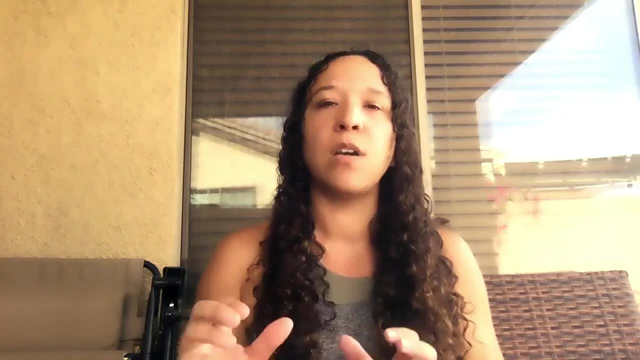 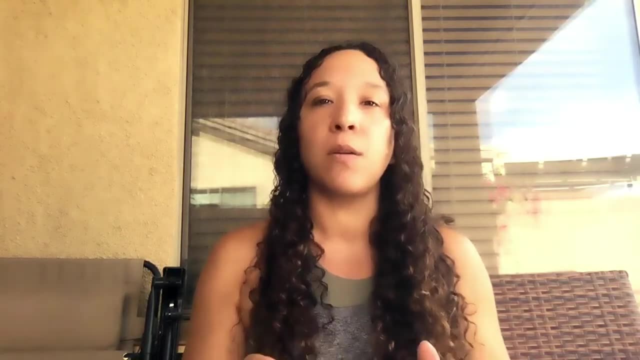 channel at least all the study videos. there is an accompanying study note that goes along with it. They're not official blog posts. I didn't edit them. They're not improper AP formatting, but you can study with them. They're free. They're a gift to youth. 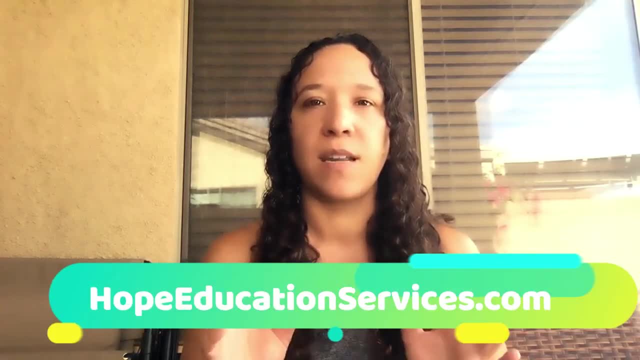 And they're on my blog, which you can find at hopeeducationservicescom. Check it out And I'll see you guys tomorrow. from the RV. 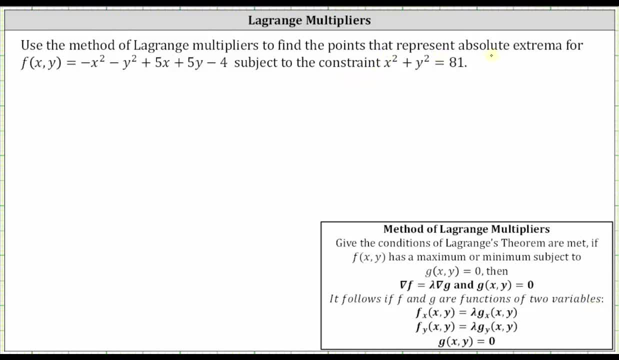 We're asked to use the method of Lagrange multipliers to find the points that represent the absolute extrema for f of x comma y, subject to the constraint: x squared plus y squared equals 81.. To use the method of Lagrange multipliers,